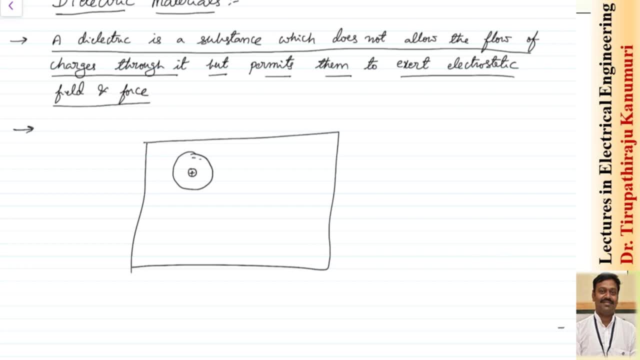 positive charge which will have proton and the neutrons, and surrounding it there will be the electrons which are orbiting in different orbits. Generally this net charge- net negative charge- will coincide with the net positive charge. Both will go inside in the center. That means effect. 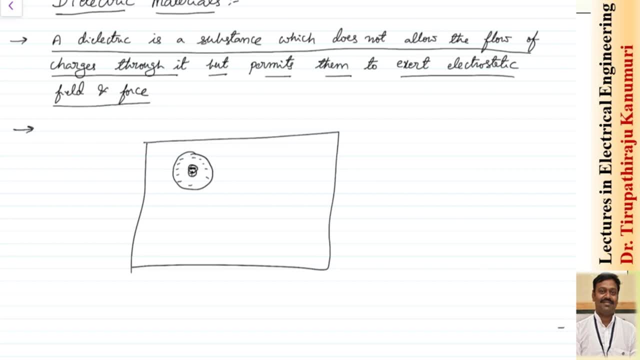 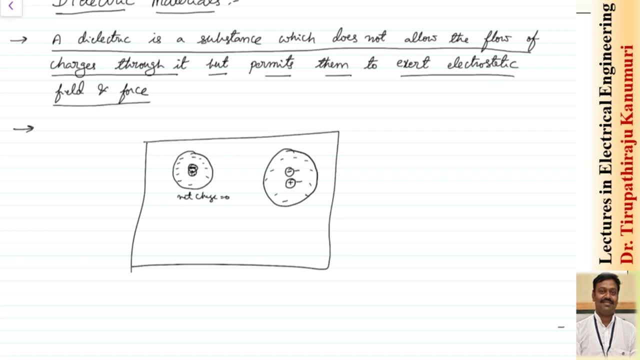 it will be shifted like this: the net negative charge will come here. there will be some small distance between them. So we call that because this is nothing but some charge, Q because this is plus charge, this is negative charge. they are separated by some distance. 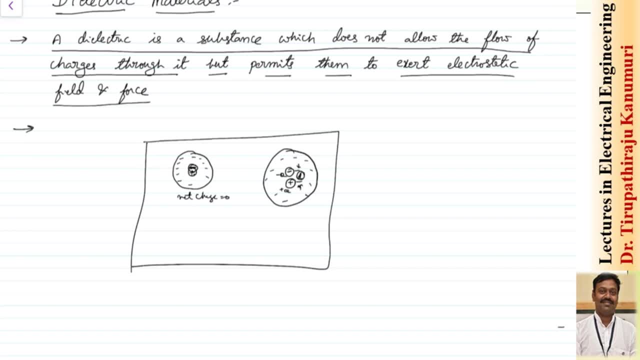 D. So we tell that there a dipole is formed, So this forms a dipole moment which is given by the dipole moment is equal to Q into D, and this Q is the any charge, that positive or the negative charge. this is the dipole moment. So the direction of this vector will 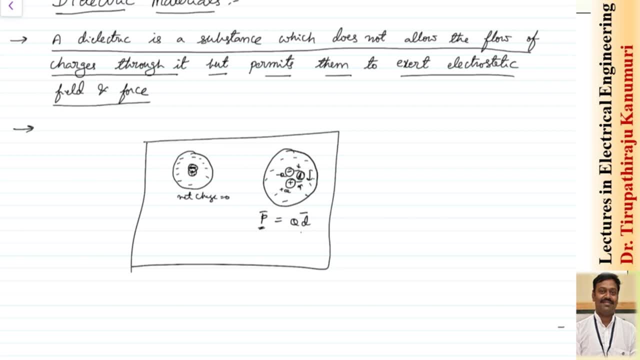 be from negative charge towards positive charge. this we have already studied. So in some type of materials it will. net charge will be 0,. in some kind of material, net charge at the atomic or molecular average is not 0,. but when you take as a set of the 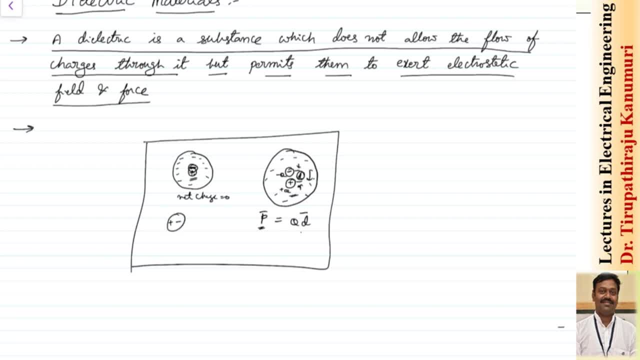 complete material. Let us assume in one material the dipole is arranged like this, another material it may be arranged like this, another material like this. they are randomly aligned So that the net dipole moment- that means, if you take in the macroscopic level, that net. 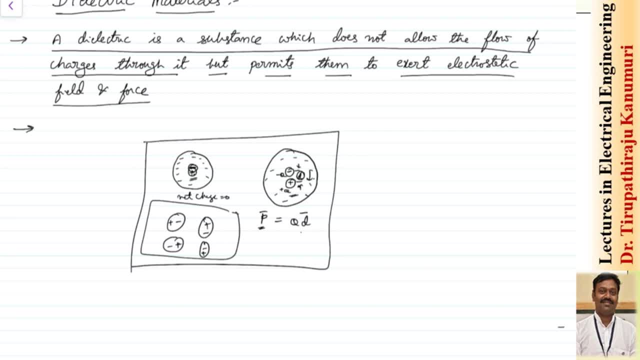 dipole moment will be equal to 0, because they cancel each other. this is what practically happens. so now, when you place the material in an electric field, it is going to experience some electrostatic force. let us see what will happen when a material is kept. 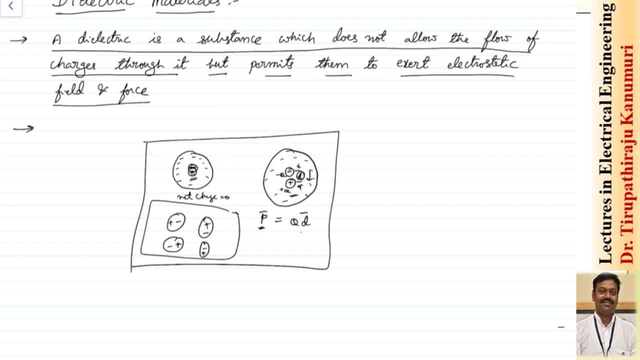 in an electric field, now based on when previously in the initial condition, whether this material is already having the dipoles or not. there are two types. the first type of material is called as this is non-polar, because it is not polarized, and the second type of material is where permanent. 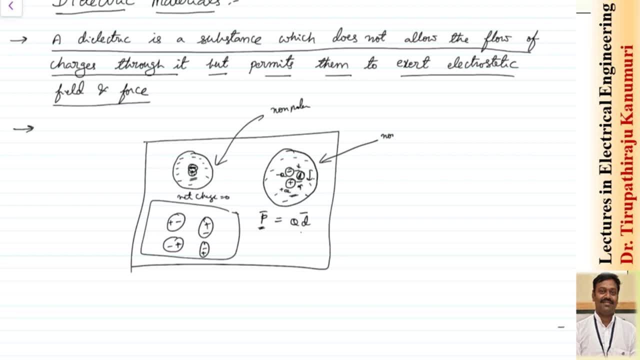 dipoles are already existing, but they are randomly aligned, so these are called as the polar. so polar example is the HCL, H2O and NH3 NACL. so these are some of the examples. and non-polar materials are, for example, H2O2, as well as CO2, etc. these type of materials there will be. they are not polarized. 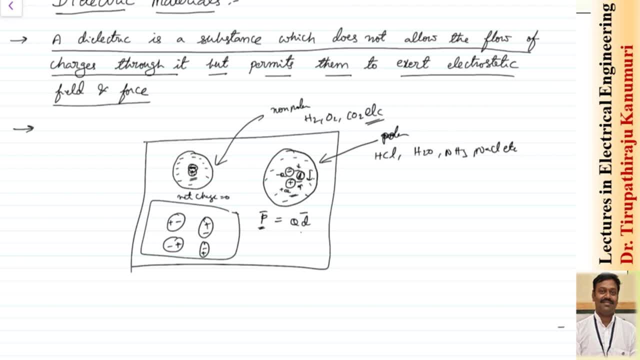 there will be no dipoles at the atomic level also or the molecular level also. but the property of the difference between the insulated and the dilated material is that they are not polarized. material is a dielectric. material is also insulator, where, when it is exposed, 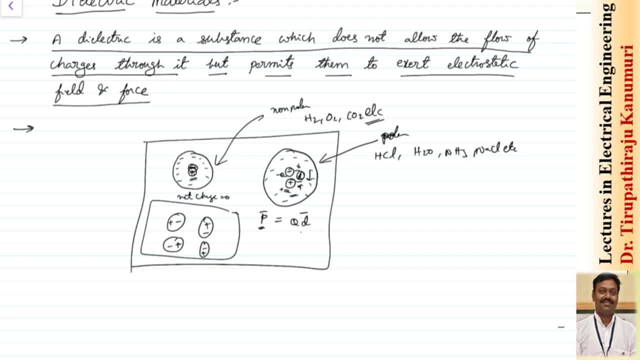 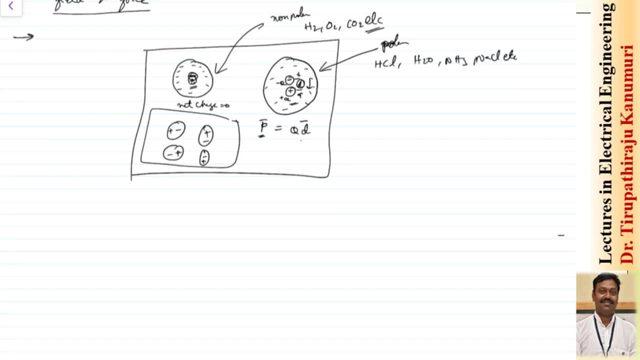 to the electric field. the dipoles will be formed in the case of dielectric materials, whereas in the case of insulators it will not be formed. that means all insulators are not dielectric materials, but all dielectric materials are insulator materials. only that means it is some insulator materials which 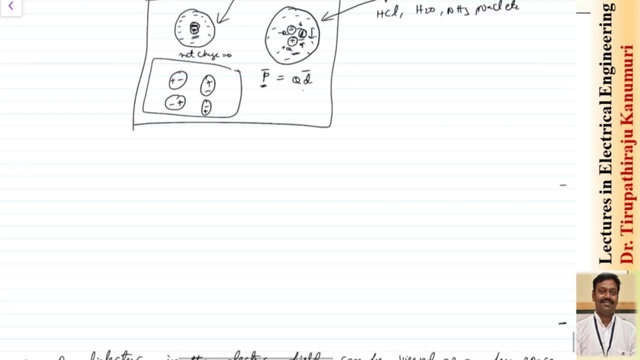 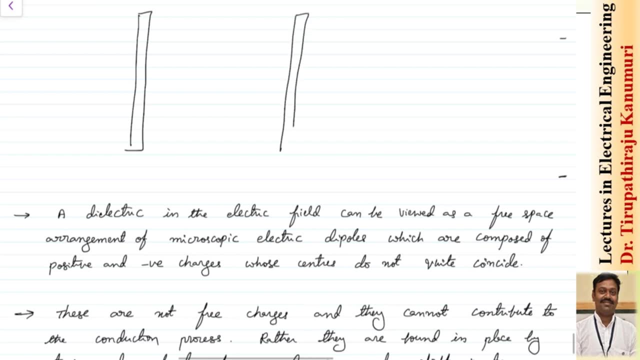 respond to external electric field we can call as the dielectric materials. so let us take, for example, I am taking a plate and between these two conductors let us assume I kept a material. that dielectric material is kept. so now this is connected to some external supply. so let us assume it is connected to some. 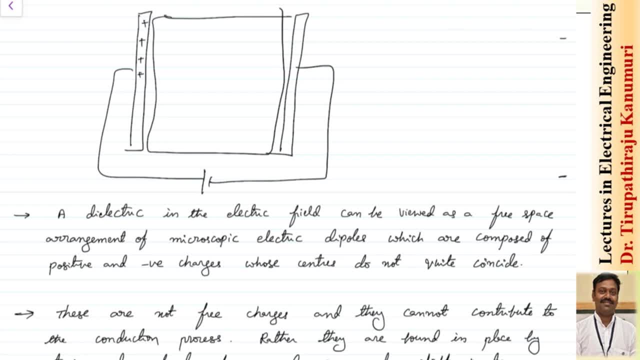 external battery. because of this the plates get charged, because we know in the conductor the surface charge density will be formed whenever the electric field is applied and here also that negative will be applied. so now, because of this the electric field is produced. let us take this electric field, this: 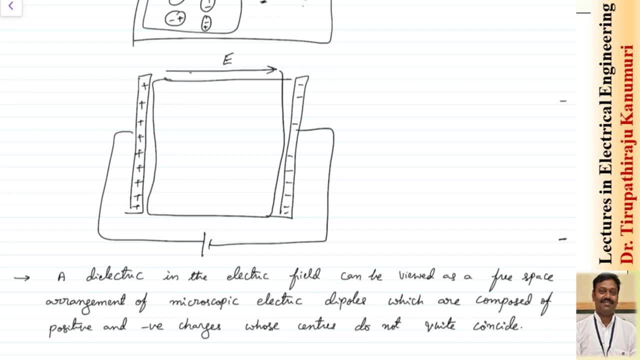 external electric field. this electric field I am representing by E. so this E naught, let us take it as E naught, that is the electric field that can be produced in free space. but when this is exposed to this electric field, what happens? whichever, the atoms are that that center of mass. like you, take this. 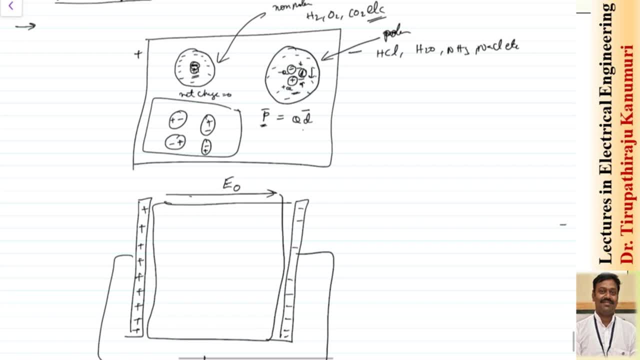 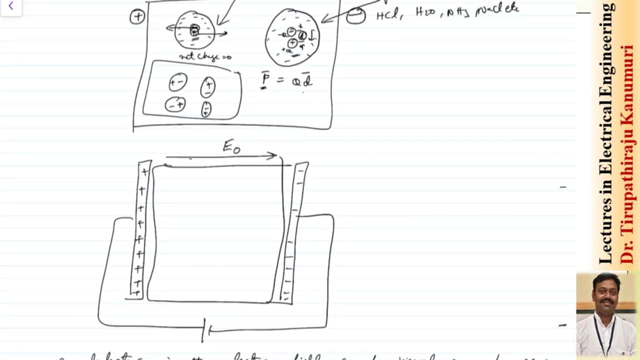 atom. this positive, because if we keep plus here, minus here, this minus will attract the positive charge or the center, and this positive or this positive terminal, this will attract the negative charge. or because of the electric field in the atom there will be different displacement will happen in. 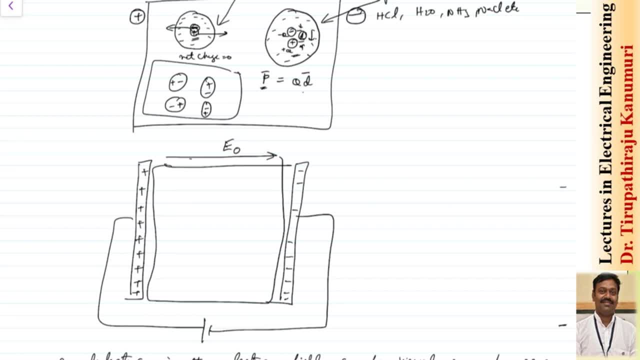 the center of charge as well as center of the positive and the negative charges. they will be displaced. so this process is called as the polarization process. this process is called as a polarization process. now what happens if you are taking this atom when this is kept in the electric field? so the net negative 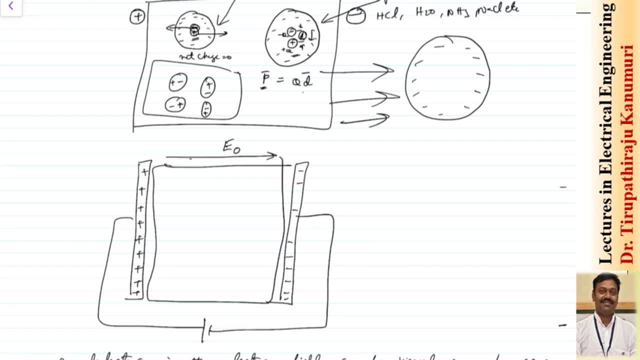 charge because different negative charges are there, so they will be attracted towards it, so that net negative charge may come here and the positive charge will be pushed away. that net positive charge may shift like this. so because of this shift, what happens? so there is a distance between them because 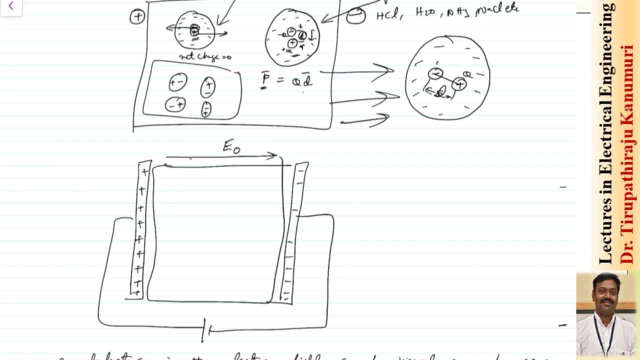 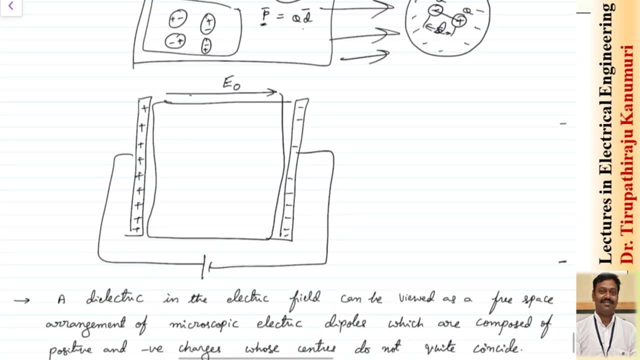 of this distance the dipole moment is formed. if this is the charge Q and one is minus Q, the dipole moment is formed at this point like that. the dipole moments are formed in each. so I am assuming that the uniform dipole moment is formed among all the elements which are kept here. so the net dipole, so they. 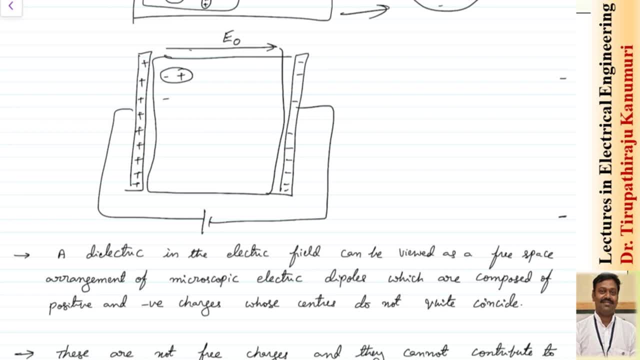 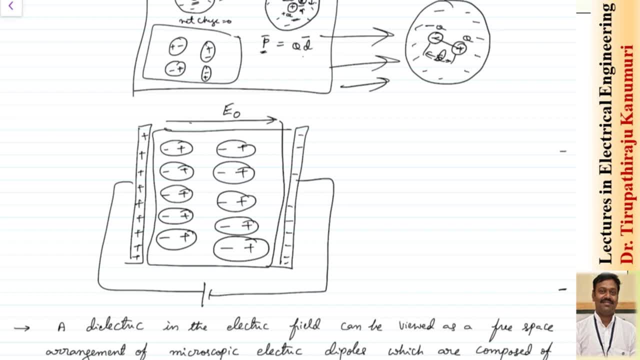 liberating out from the valence band. actually they are just rearranging themselves because of the application of the external field, or we can tell that these charges that are formed, this positive and the negative charge- they are bound in the position. they cannot be completely liberated out. that's why 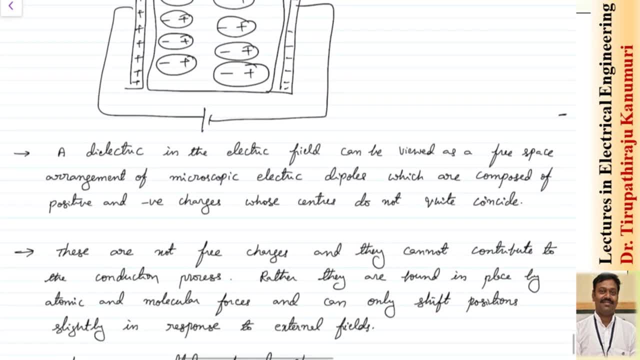 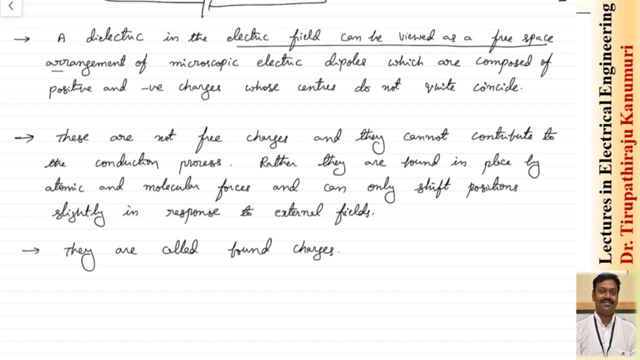 these charges are called as bounded charges. so I can summarize that what we observed till now in a dielectric in electric field can be used as a free space arrangement of micro electric dipoles which are composed of positive and negative charges whose centers do not quite coincide. the centers are displaced, so these are not. 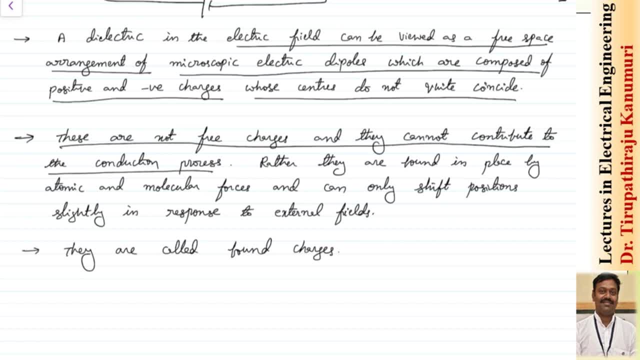 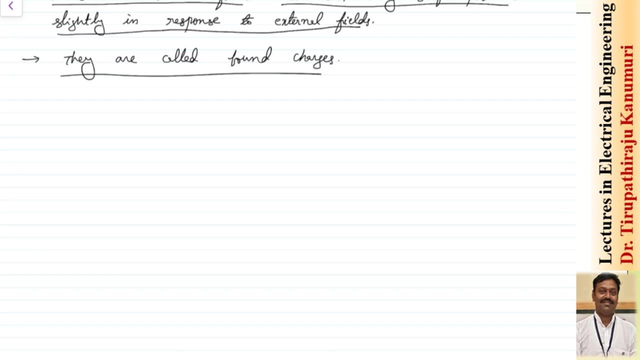 free charges and they cannot contribute to the conduction process. rather, they are bound in place by atomic and molecular forces and can only shift the position slightly in response to the electric fields. so that's why we can call them as the bound charges. we can call them as the bound charges now, as a 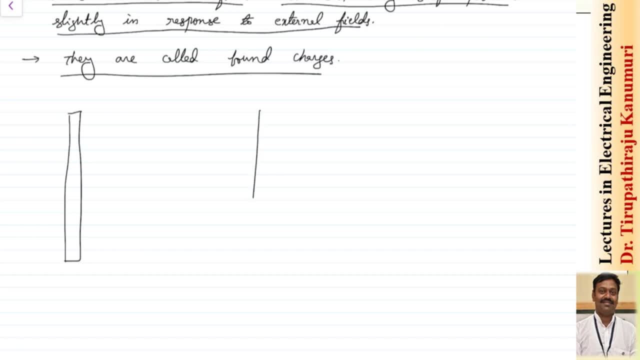 result of this, what happens? so let us take the plate here. let us take another plate here. so in this plate, let us assume here it is positively charged by connecting an external supply. so here it is the negative charge due to the external supply. so now, whichever material let us, 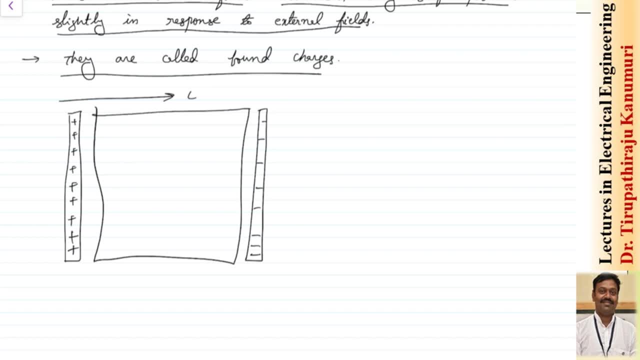 assume some dielectric material is there. so because of the external field, the electric field that is produced is E naught. that electric field produced is equal to E naught. so let us see under different conditions. if E naught is there, let us keep in the free space. in the free space, whatever the 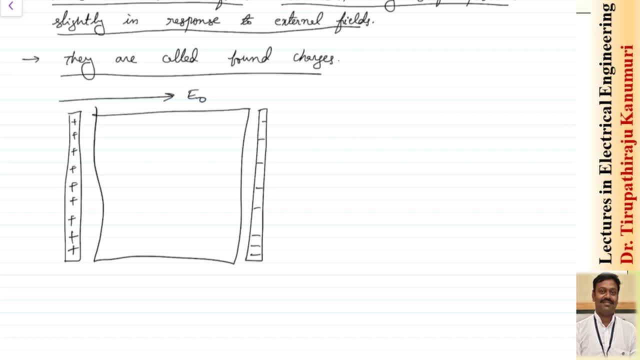 electric field is produced, the same electric will pass through the free space. So we can tell that inside, whatever is inside, that means between these two spaces the electric field will be same as E naught, But if you take for the case of the conductor. so this I am just 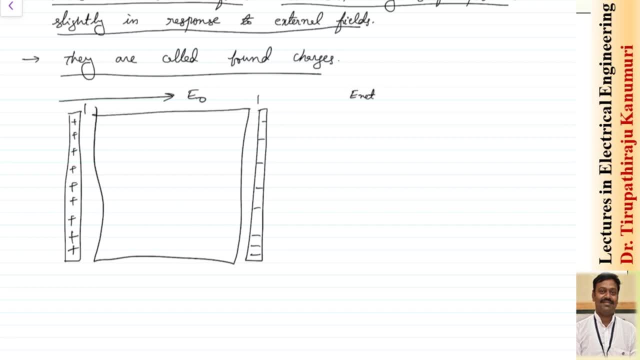 defining by the term. let us take it as the net electric field that is inside is defined by some E naught divided by some constant k. Or we can tell that some constant k I am defining by E naught divided by the net electric field inside. So this is defined by the dielectric constant. 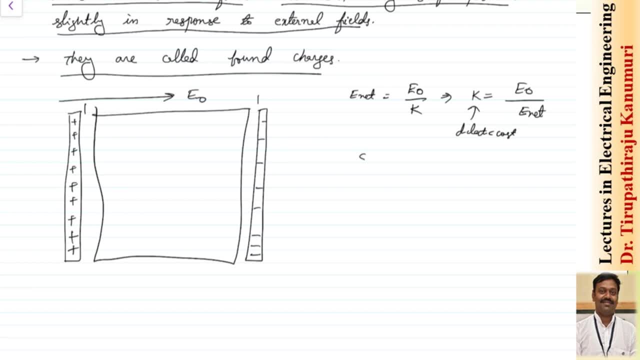 dielectric constant. So if you take the free space, in the case of free space, so whatever the electric field is given, the same electric field will pass in the net also, inside the space also. So E net is equal to E naught. So we can tell that k will be equal to 0.. Now let us take 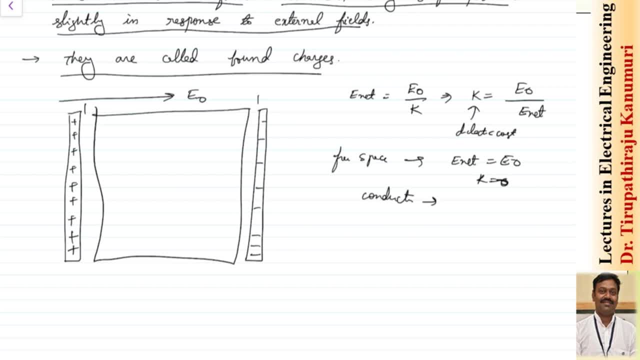 for the case of conductors. We have seen in the conductors that whenever the electric field is applied, all the electrons or all the charges will be displaced or shifted to the boundary. So they will be attached to one of the surfaces And only there. 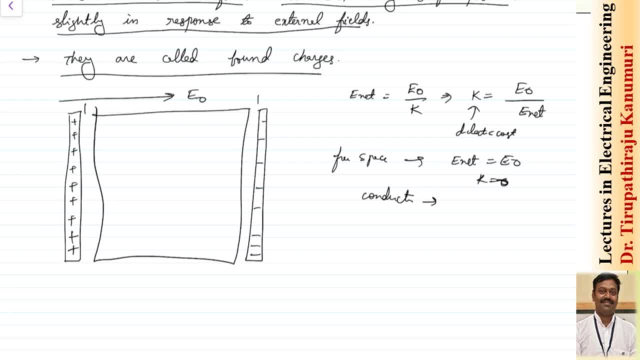 the surface will be attached to one of the surfaces. So they will be attached to one of the surfaces And only there the surface charge density will form. And inside because of the surface charge. we have seen that the electric field produced because of the surface charges. 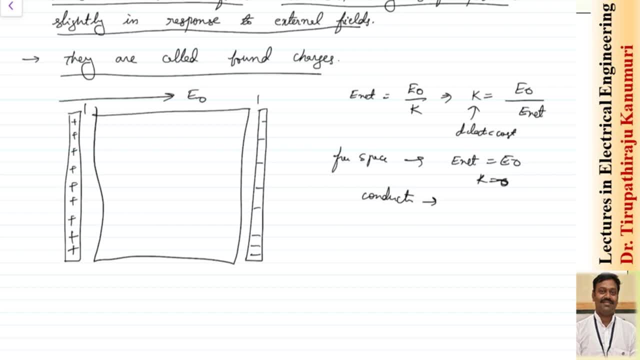 will oppose the cause. The cause is E naught, So the net electric field inside the conductor will be equal to 0. This is already seen in the conductors. E net is equal to 0. So from this, if you calculate the k value, k value will be E naught divided by 0. So k will become equal to. 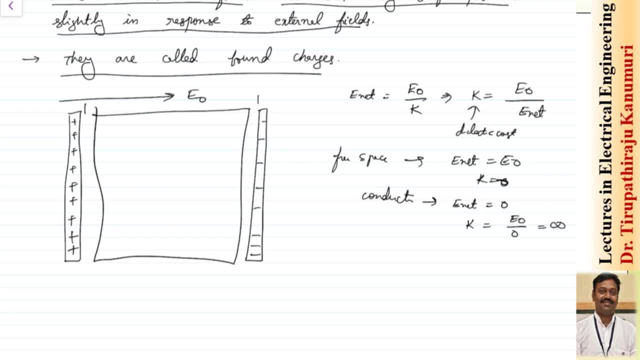 infinite. So if you go for the case of dielectric materials- the dielectric materials- this E naught will not be equal to 0.. E is a non-zero value, But we know that E naught will be less than the. 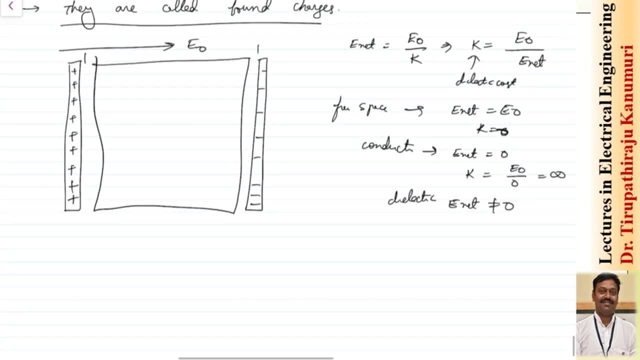 what is electric field applied? because net electric field will be decreased there. So we can tell: the value of k is equal to E naught divided by E net. So this will always be greater than 1.. So we can tell that for a dielectric material the value of k is greater than 1. Whereas in the case of free 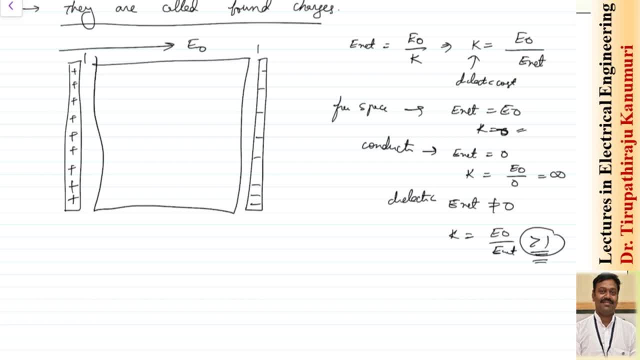 space. so k will be equal to 0. It is not going to affect anything In the case of conductor. it will be infinite. So in some materials it will not be equal to 0 or the infinite. It will be intermediate between them which will be greater than 1.. These materials we can call 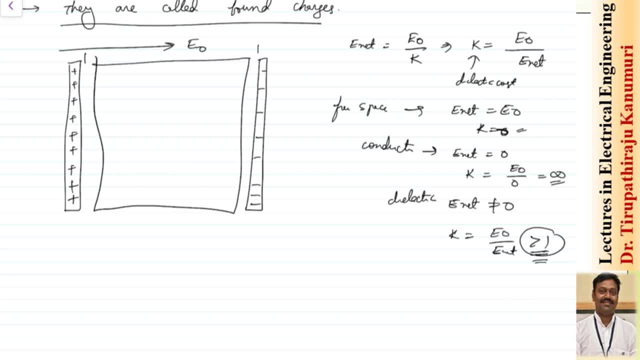 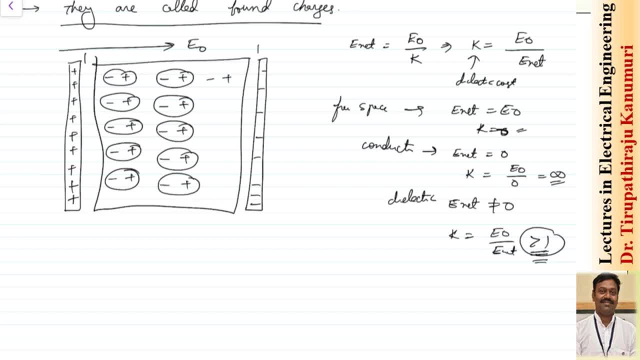 Only that is the difference between them. So I am just representing here. So because of this, the net electric field is displaced, The net electric field is changed. So let us try to analyze that. So practically whatever the E net that comes- because you 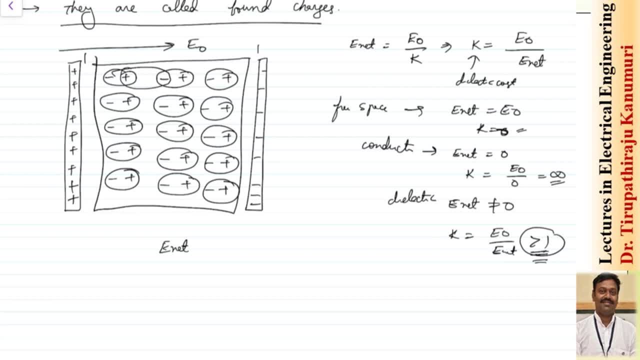 can see here. this plus minus. these are nearby, So this we can take as cancelled. This also will be nearby. this also nearby, this also nearby, this also nearby. All the dipoles are aligned like this You can see here. So these things we can cancel in the center. 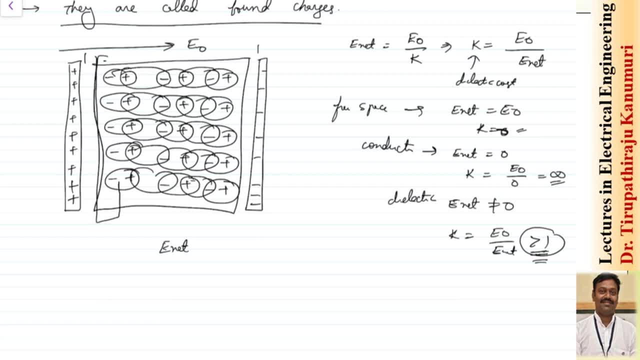 We can tell the net effect will be: whatever the charges are on the surface, these are negative. Whatever charges are coming here, these I can call as positive or otherwise. we can tell that, as all are adding to each other, we can tell a dipole moment is formed. 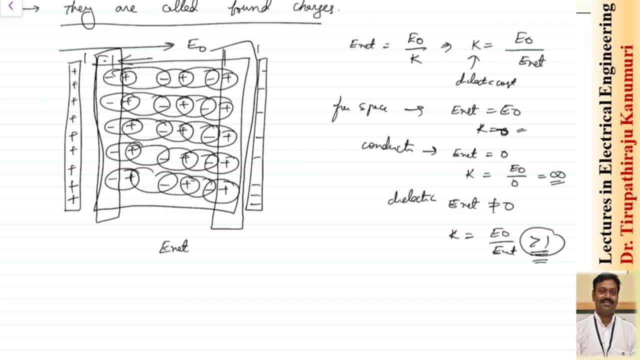 or a dipole is formed with the gap. what is the distance between these two? Let us assume the distance between these two I am representing by d. I can just represent this entire thing by having a positive and a negative charge, which are displaced by the distance. d because 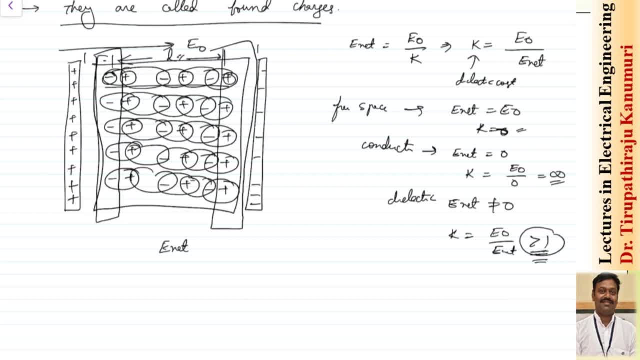 they will add to each other. So in that form I can represent. So as a result of this, because this positive charge is here and negative charge is here, So I can say that this is positive charge which is here, So this produces some electric field. This electric field will. 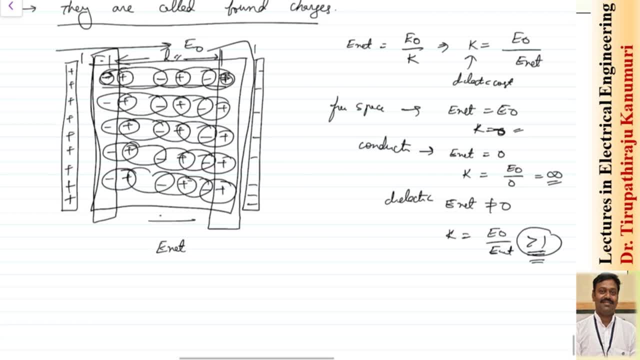 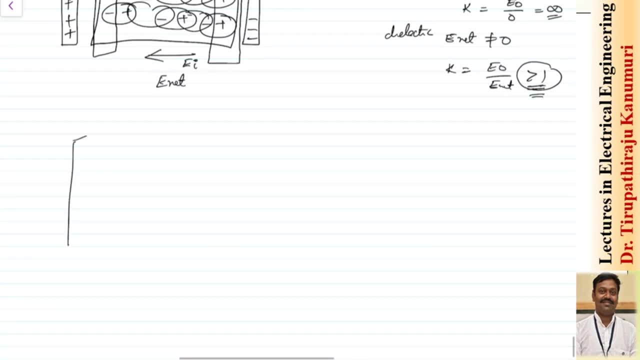 be in the opposite direction to E naught. That means this will produce some electric field, So that I am representing by E i. The induced electric field will be from positive charge to the negative charge. So let me represent that here: plus, plus, plus So. 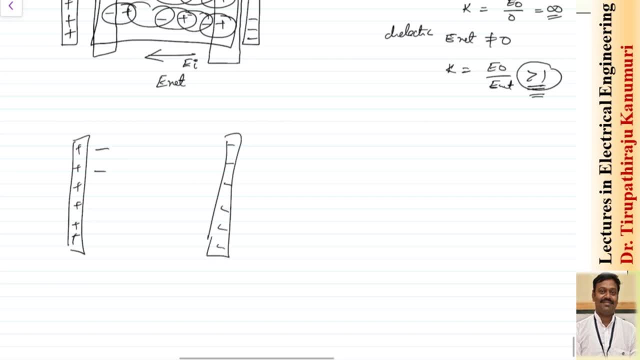 here it is my plate: minus minus, minus. So here the negative charge is there and here the positive charges are there. So, because of this, what happens? Whatever the E naught, that is applied because of this thing, because from positive to negative there will be some charge. that is. 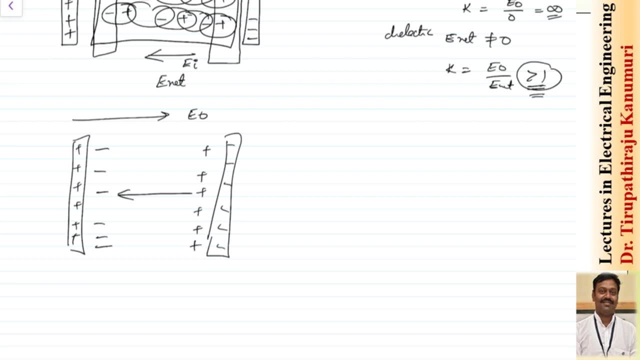 produced because the electric field will be produced because of these bound charges. So this electric field I am taking as my induced electric field, So we can tell the net electric field inside the dielectric material will be the electric field that is applied and this induced. 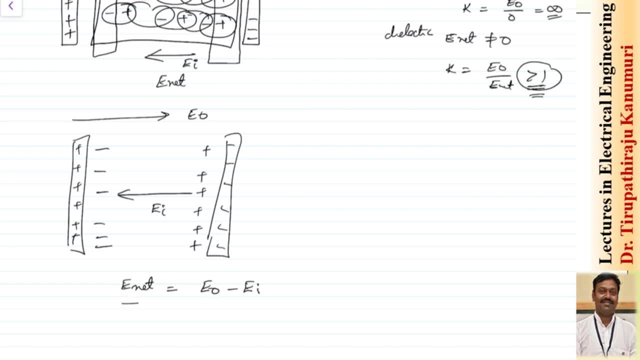 electric field is opposing that one. So it will be E naught minus E I. This will be your net electric field that is coming. So let us try to analyze this further So we can tell that the polarization p is nothing but the dipole moment per unit volume. So let us assume n. 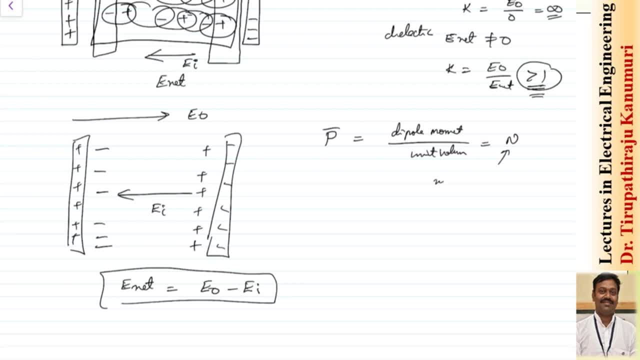 number of atoms are there per unit volume. These are number of atoms per unit volume and let us assume small p is the dipole moment. dipole moment. So this is induced, So we can call it as induced dipole moment. So let us take the example a capacitor is. 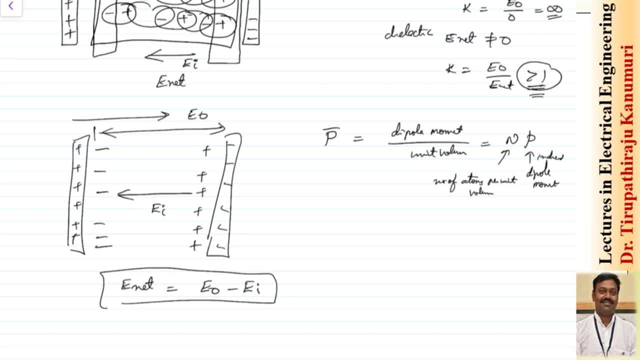 formed or something is formed, a dielectric material is kept Here. the gap between them I am representing by the distance as d, and let us assume the surface of this plate is having a surface area of A, or we can tell that the volume of the material that is kept inside the electric 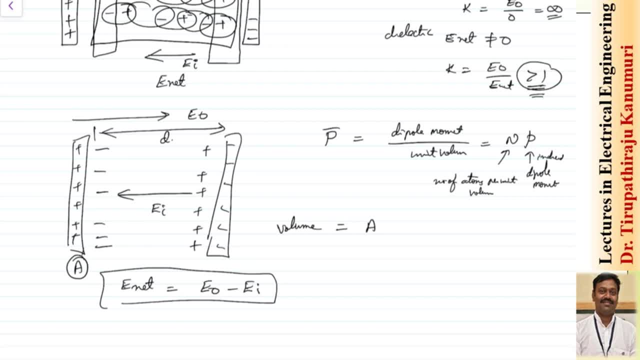 field will be the area. that means in the side. that is multiplied by the distance, that means two sides, whatever is the gap between these two sides, like this, So we can tell the polarization in this case. So we can tell the polarization in this case. So we can tell the polarization in this. 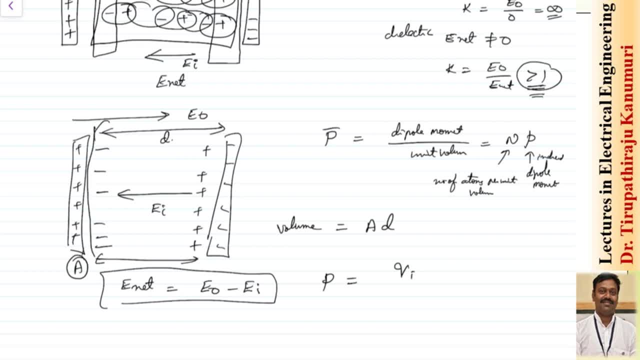 case will be the qi. qi is the total charge that is accumulated in any one side, either this side or this side. This total qi, this I am multiplying with the distance d, because that gives the dipole, dipole moment, So divided by the volume, volume is A multiplied by d. So this I can write as: 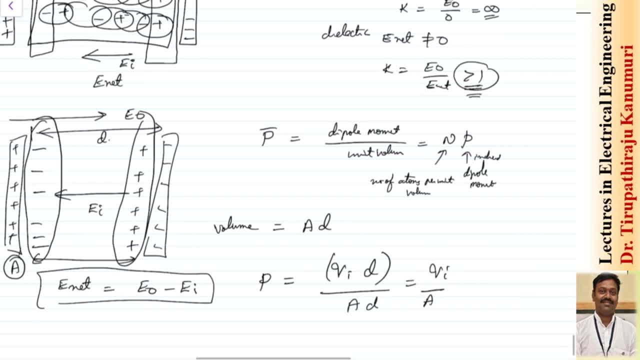 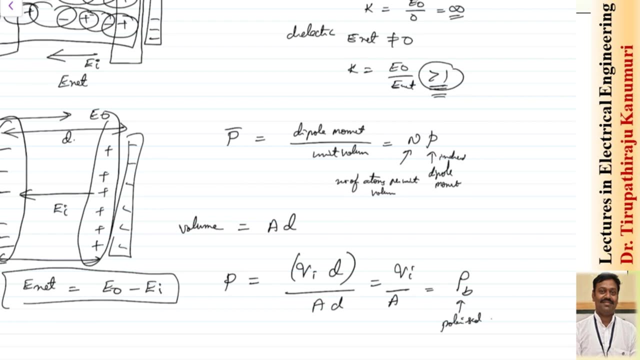 qi divided by A, that means this is charge per unit area. We know the charge per unit area is represented by charge density. So charge density I am representing by rho suffix b. This I am writing by the name polarized bound charge density because it is bounded. That is why 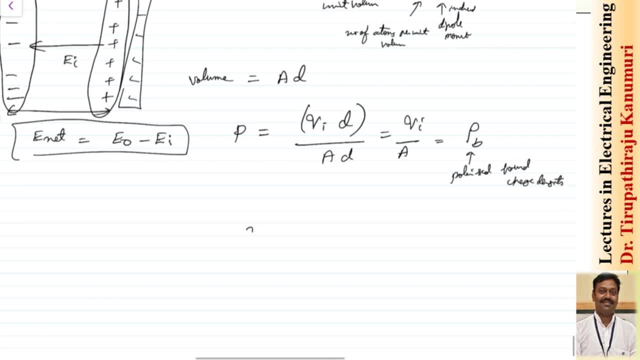 I am representing with rho b, or I can represent this as some vector n dot product with the polarization. This gives the value of rho b. So this indicates the unit vector. So this unit vector. we know that always in a polarization we can do this. So this is the unit vector. So this. 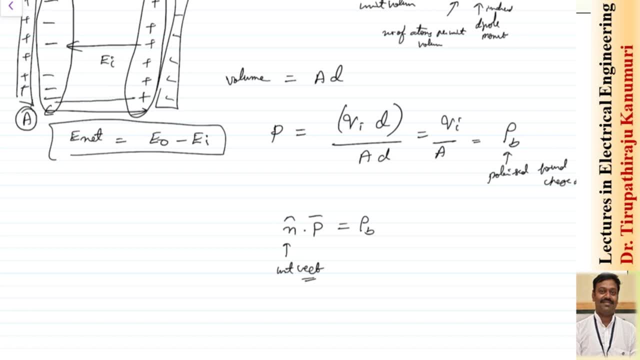 can define the polarization we give from the direction, from negative to the positive direction. So this is my polarization. p Polarization vector will be always directed from negative to the positive, You agree with me. So let us try to calculate the net electric field So you can tell. 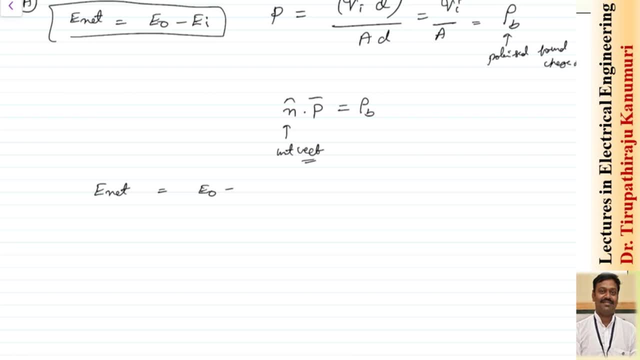 the net electric field will be equal to the charge that is given. that means that is given minus what is produced because of this bounded charges, What is produced because of the bounded charges or the induced charges. So let us take it as ei. So this I can represent as 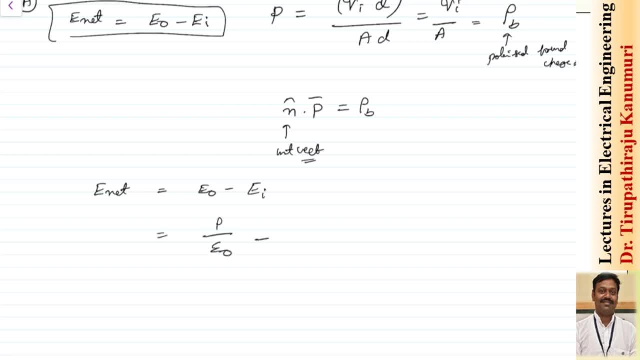 rho by epsilon naught minus rho b. that means bounded charges by epsilon naught, because we know that divergence of d is equal to the charge enclosed divergence of d from that. we can define this So we can tell that the net charge will be rho by epsilon naught minus. 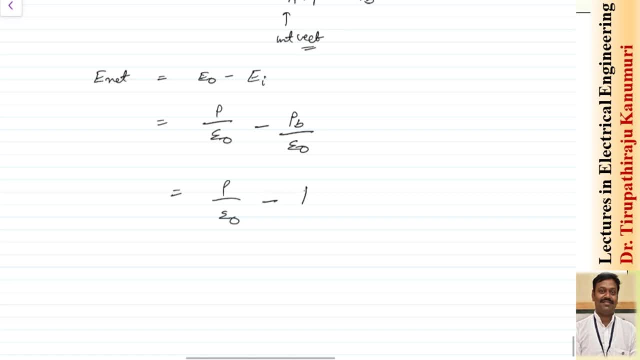 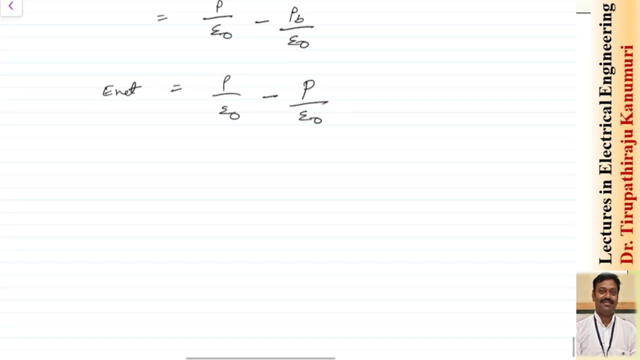 this will become rho by epsilon naught minus the polarization p by epsilon naught. This is the value of e net. This is the value of net electric field. So now it is a very. it is observed that the polarization, whichever is coming, that is proportional to the net. 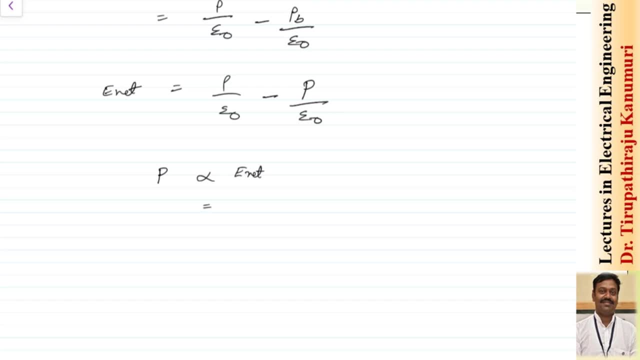 value of the electric field that is inside, or if you remove this proportionality constant. this can be given by. this is given by chi. This is generally called as chi. So chi into epsilon naught into that net electric field, or we can tell that the net electric field. 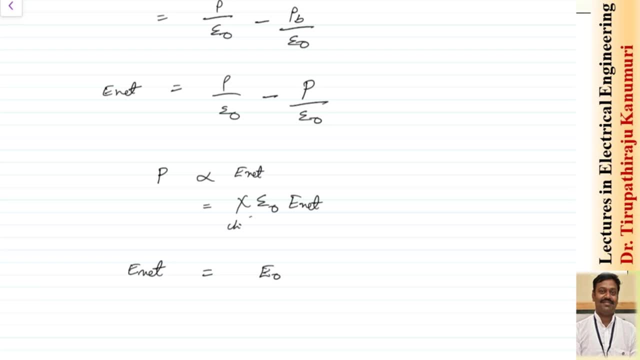 that is produced will be the e naught. that means the electric field that is given minus because the polarization is opposite direction to the electric field. So this will be p divided by epsilon naught. So we have to take it as P by epsilon naught, because the induced 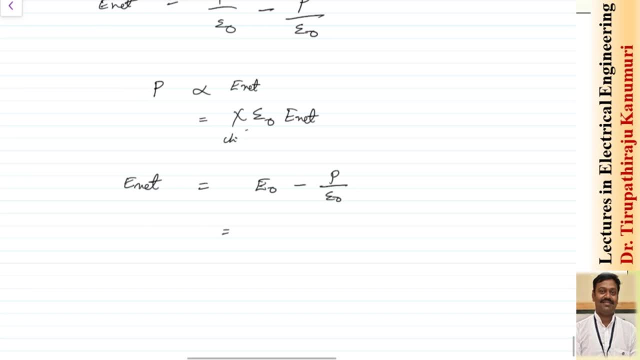 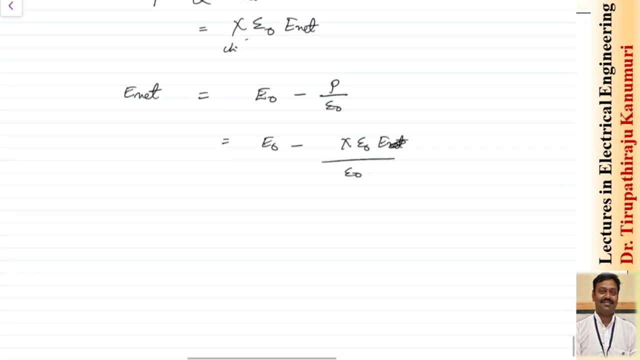 charge is opposing it, or induced electric field is opposing this. So this I can write as E naught minus that P by epsilon naught. that P I can write as chi into epsilon naught, into E net divided by epsilon naught, or this I can, I am writing it as induced values. So 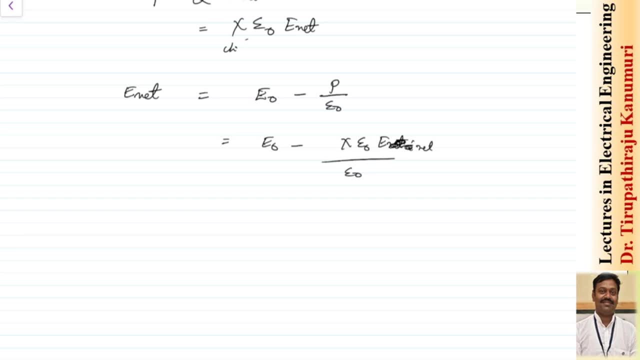 this will be depending on net value only, right E net value or the net value or the resultant value. So from this I can rearrange this one So I can bring to the second side E net plus some chi times of epsilon naught into E net. divided by epsilon naught is equal. 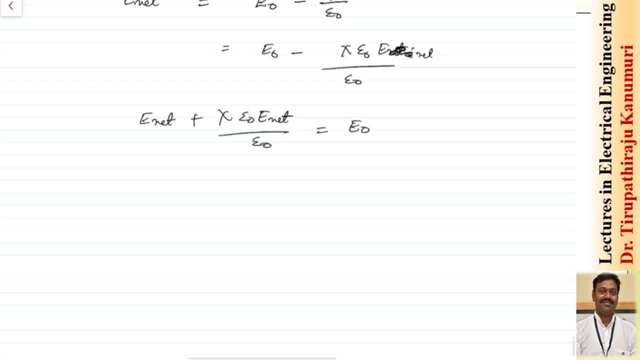 to E naught. This is what we obtain. So this I can further simplify: epsilon naught, E net, this I can, multiplied by 1 plus chi is equal to epsilon naught into E naught. So this 1 plus chi. 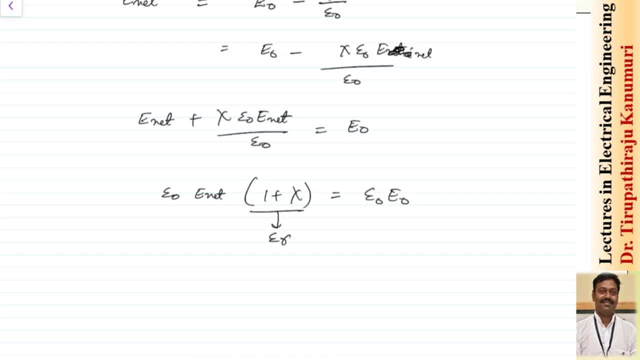 So this 1 plus chi is called as the relative permittivity, or epsilon r. This is called as relative permittivity, or epsilon r: This is called as relative permittivity. This is called as relative permittivity. So we can write this as: epsilon naught epsilon r into: 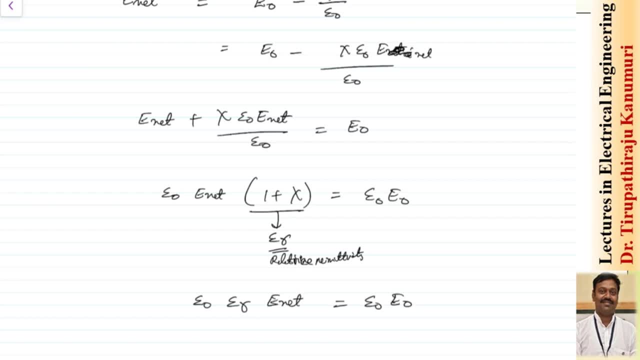 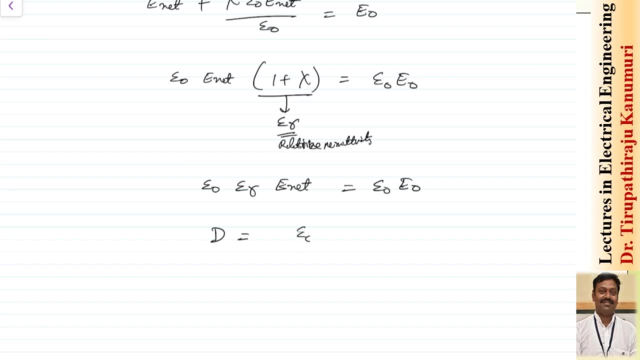 E net is equal to epsilon naught into E naught. So we know that epsilon naught, E naught because nothing but the flux density in the free zone. So one more using the velocity space, So we can tell that D is equal to epsilon naught. 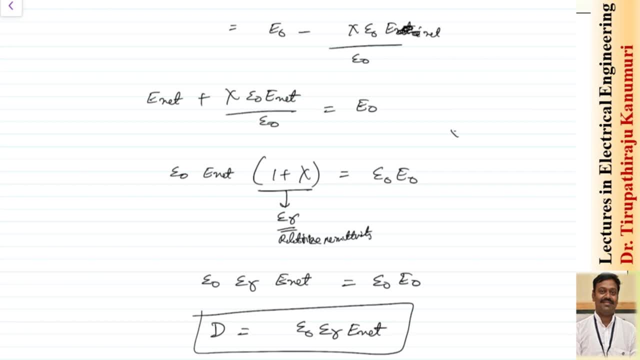 into epsilon r, into the net electric field. This is the relationship. Let us now see what is called this chi. chi is called as the susceptibility. So this susceptibility indicates how much of your material is susceptible to the electric field. That means if your material is more susceptible, then more electric field it will. 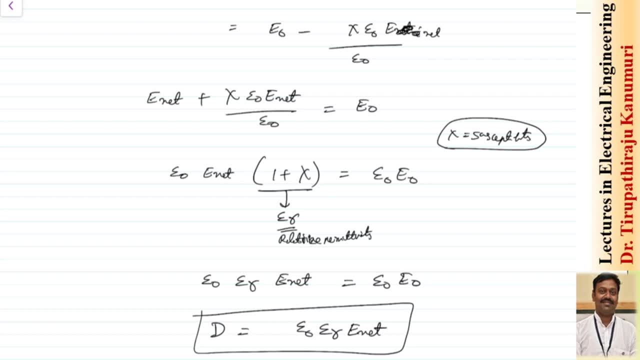 have more dipoles. if it is less susceptible, it will have less dipoles or less dipole moments. That is the material sensitivity. Potentially, this is not going to work, which is why we have more dipoles, The dipoles chocolates. more So if these dipoles are more susceptible to dipoles, are going to have deep dipoles, More dipoles or even less dipoles. Now, what happens eventually? if there is more dipoles, what happens? 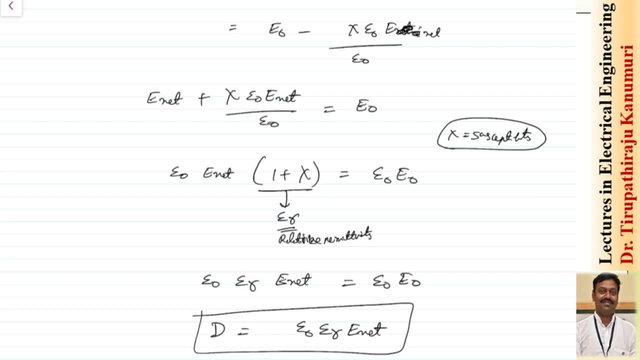 moments. that is the meaning of this susceptibility. i hope the susceptibility is clear to you. now we have defined that dielectric constant, that k is equal to that value of e naught divided by e net. e naught divided by e net. so we got the value of the e net from this equation. so this i can write: 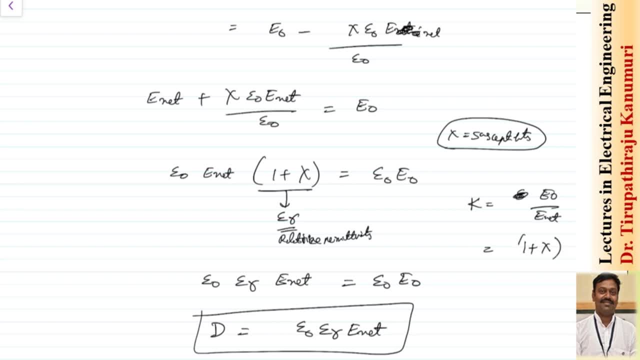 as e naught by e net. if you calculate this will nothing but one plus psi value, because e naught, because this is e naught divided by e net. from this relationship you can get as one plus psi. so we can tell this that one plus psi is nothing but dielectric constant, or sometimes it is also. 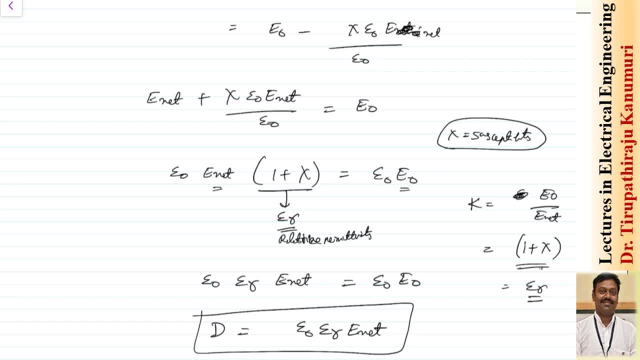 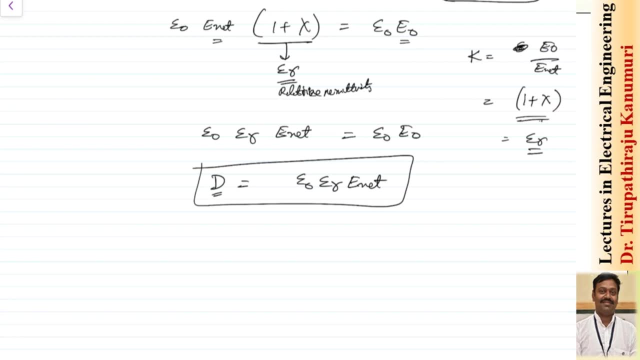 represented by the term epsilon r. so i think this is clear to you. so we can tell that in a dielectric material the relationship between the free charge density and the charge density that happens in dielectric material is: d is equal to epsilon naught into epsilon r, into e net. so we can tell. 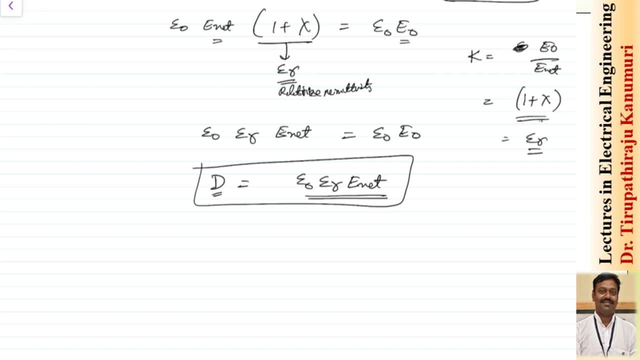 that whenever the electric field is produced, some of the electric field, because some energy is absorbed by your dielectric material and that will be stored in the form of potential energy, and when you connect your terminals back to something where the conducting path, where it can return back its 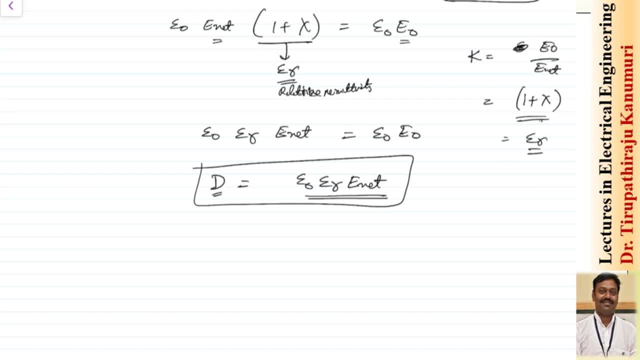 energy. it will dissipate the energy back. so in the coming classes we are going to discuss about how this is going to be used in the principle of the capacitor and how the capacitor works. i hope this the complete concept of dielectric material. what will happen when it is kept in a 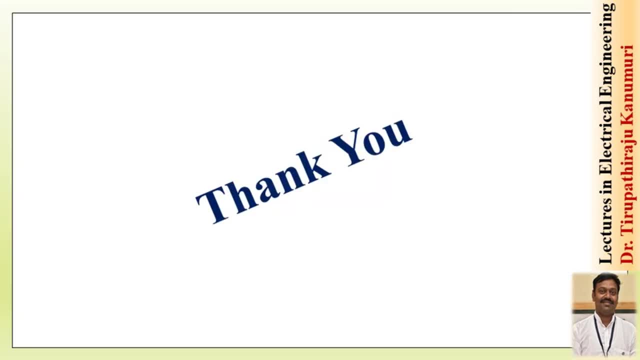 electric field is completely clear to you. if you still have any queries, you can leave your comments in the comment section below. i will answer to your queries from there, thank you. thank you very much.